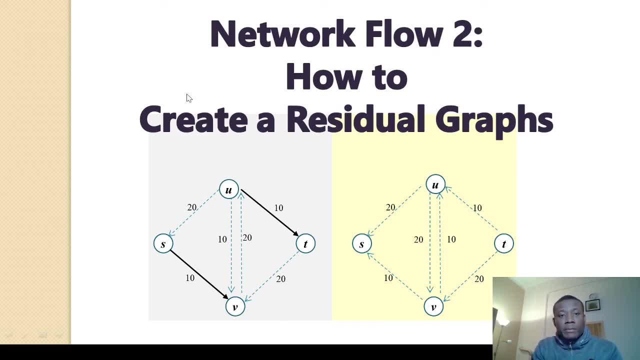 All right, today we are going to be talking about how to create a residual graph. Residual graphs is a topic in network flow, which is a very important subject in computer science. So if you're actually not a computer science person or you don't want to learn about this, you can actually skip. 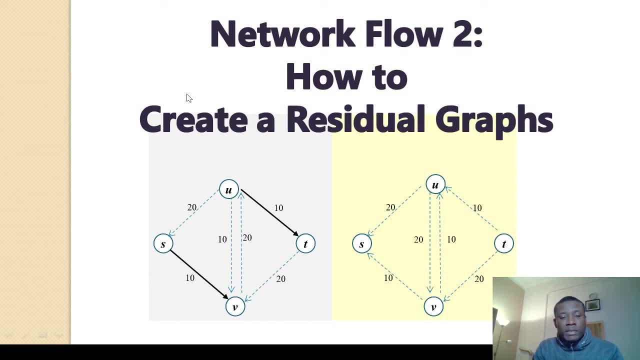 But I think it's necessary for every IT person to know about flow networks or network flow. It's simply how to make more efficient use of the network capacity, be it a communication network, electronics network, computer network and so on. So one way to do that is to create a residual graph. 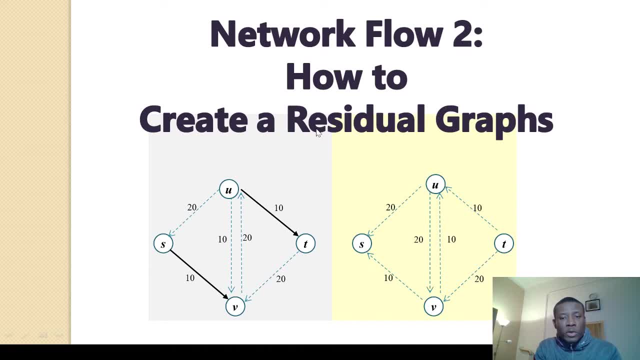 Residual graph is simply a sub-network from the existing network, For instance, this is the original network. This is the residual graph, And residual graphs helps you to see how you can improve Or what links in the network you can actually improve the flow or the traffic. 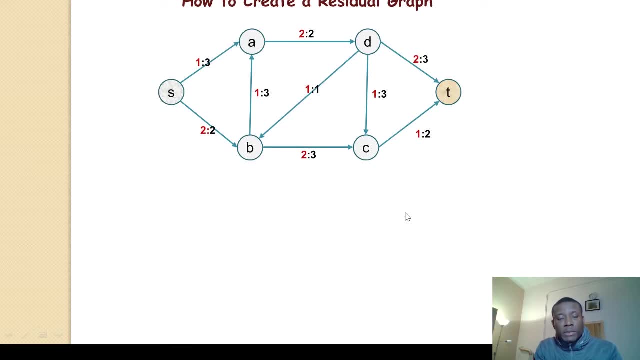 So let's go ahead to look at the procedure for creating a residual graph in a flow network. I also want to remind you to subscribe to my channel by clicking in the subscribe button below this video, So that you get updates when I make new lessons and also. 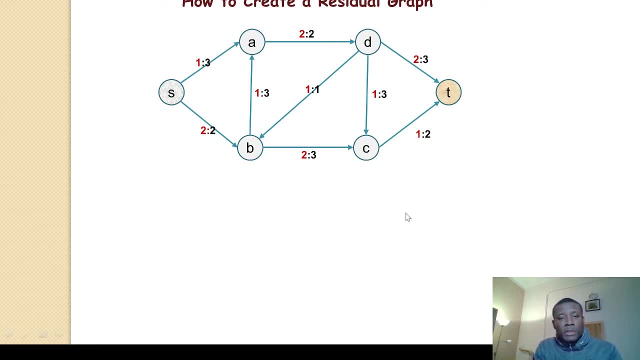 do let me know. if there is any topic you like me to discuss or treat, or some observation you find that you'd like me to clarify, leave in the comments below And I'll get back to you. So, in creating a residual graph, there are some rules that you need to apply. 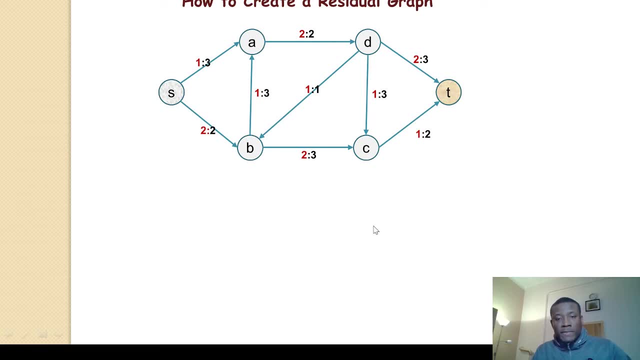 Rule number one: the nodes in the original graph is exactly the same set of nodes in the residual graph. So get this clear. the rule number one: this set of nodes one, S A, B, D, C, T or S A, B, C, D T- is exactly the same set of nodes in the residual graph. 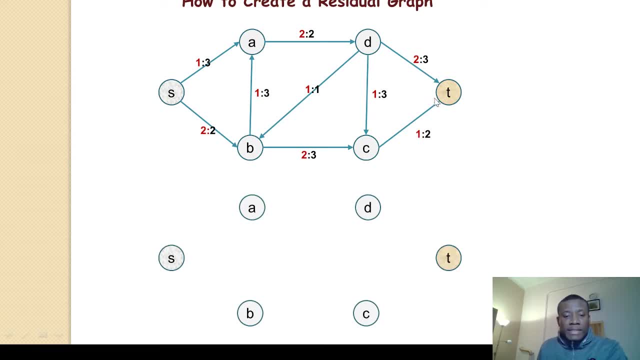 So let's start with that. So that is the starting point for creating a residual graph. Now there is another rule called the forward edge rule and the backward edge rule, right? So how does it apply? It means that the first set of edges you need to consider is the edges that have 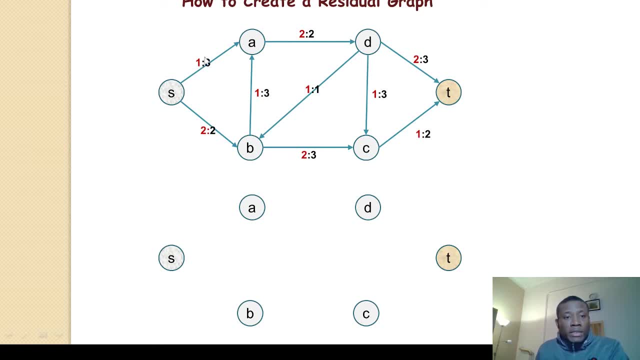 capacities that are not completely used. So if we have three being the capacity of this edge and we have one to be the flow on this edge, currently it means it's not fully used. So edges like this provide two edges in the residual graph. 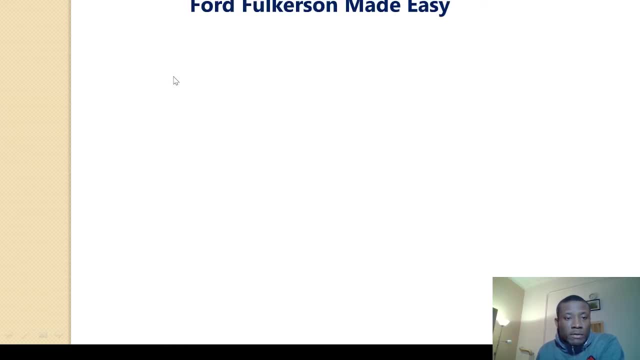 So one of the edges means you can actually push additional flow. oh sorry, you can actually push additional traffic in this case is 3-1, which is 2, you can push 2 forward And you can push 2 back. 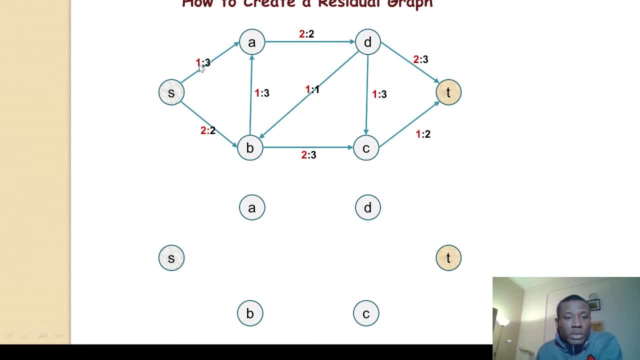 can also undo the already existing flow, which is one. we can actually remove it. so it means you have a backward edge of one and a forward edge of two. so let's go ahead to do that. if you actually find this difficult, challenging, just pause the video and see how you can understand it a bit later. let me take another color of. 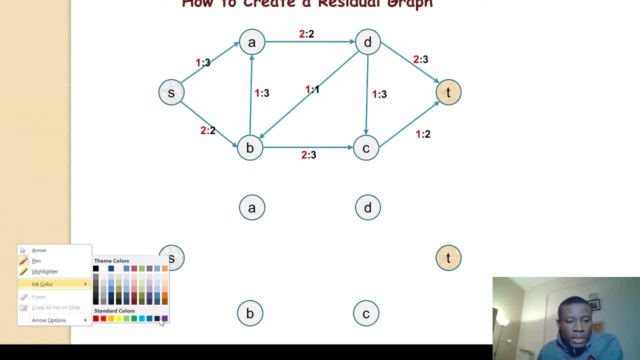 paint. maybe I'll use this color alright. so I'm adding a forward edge of how many of two, because you can push two more across. so a forward edge of two. so what these numbers are, they're actually not flows, but they are called residual. it's called residual capacity and we add a backward edge of one. 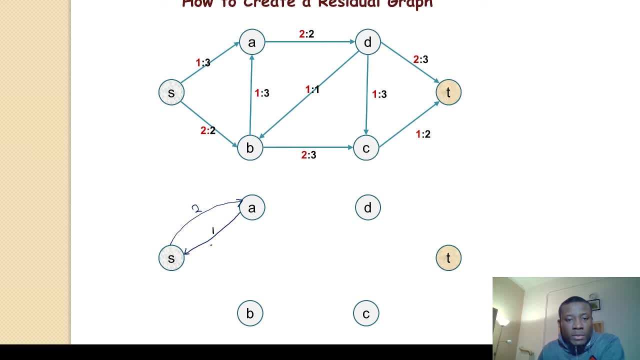 meaning that we can undo the existing one, so to add one. so let's consider the one from A to D. so a forward edge of two or a backward edge of two. this is called a saturated edge. so, saturated edge, you can add additional flow in the same direction. 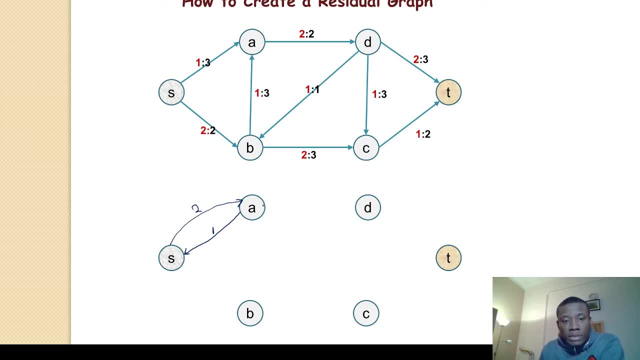 you can only move flow backwards in the opposite direction. so let's add a backward edge from here and we can undo the existing flow of two right. so we have two already and it's saturated. we can add anything further we can. we can only undo. so we add a backward edge from d to a. 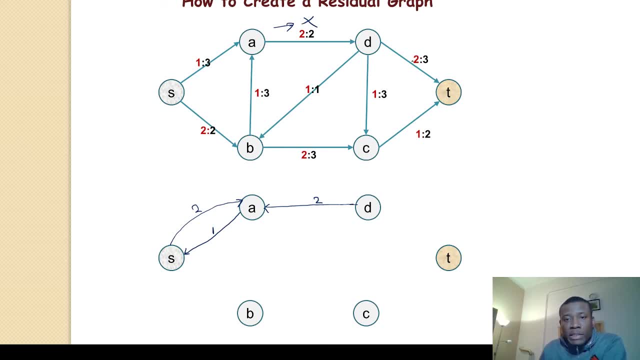 let's consider this here we have 2- 3, meaning that we have a flow of 2 already, so we can undo it by adding a backwards edge, right? so let's add a backboard edge of 2 and we can add additional forward traffic of 1. 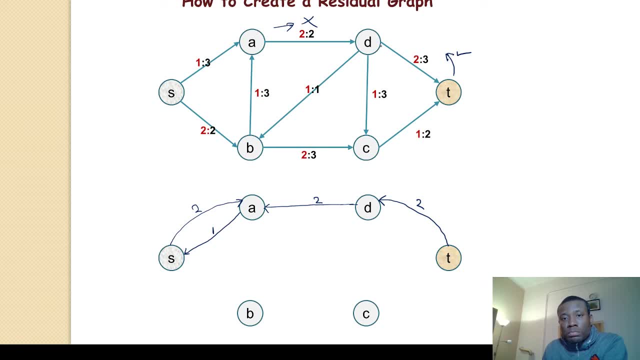 because we need one more to make this saturated. So simply three minus two is one, So we can just add it in this way. Okay, one right. So I hope you are following. So let's look at S to B. So here is saturated. 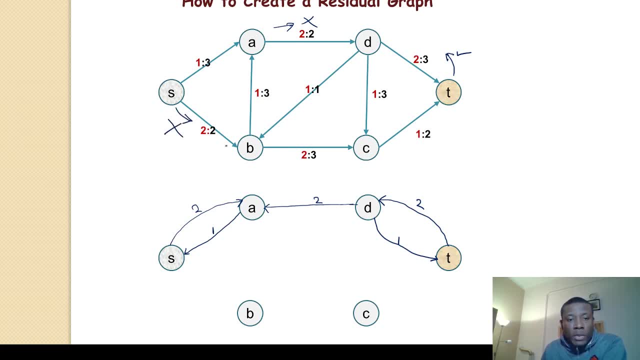 We can't push anything further. no, we can't. So we can only push backwards right. Good, by removing this two. that is already existing, So let's add a backward edge. Good. So let's consider B to A, B to A. 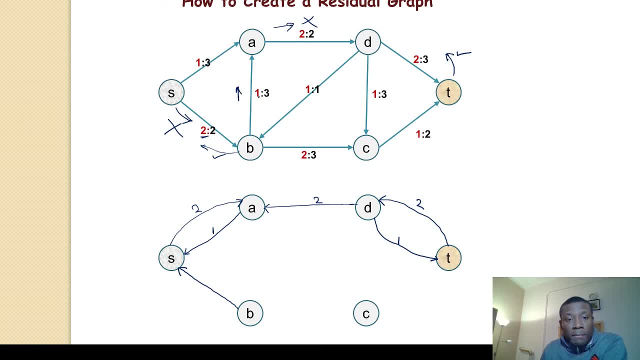 So here we have a flow of one, a capacity of three, meaning that we can add two more flow in the same direction. So let's add: okay, this is not very straight, So we can add two more in the same direction, like this: two: 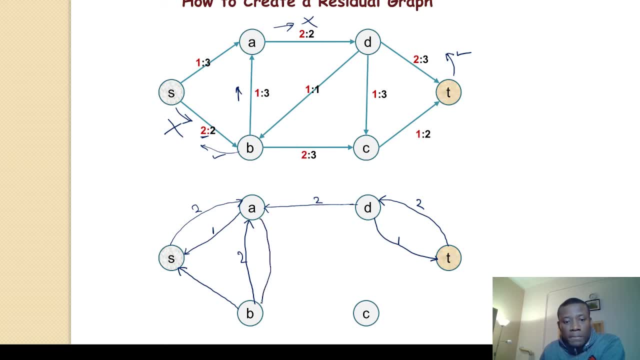 And we can remove the one that's already there. So we undo the one by sending to backwards of one right. So let's consider B to C. Here we have two existing flow, so we can remove it by putting a backward edge in this place. 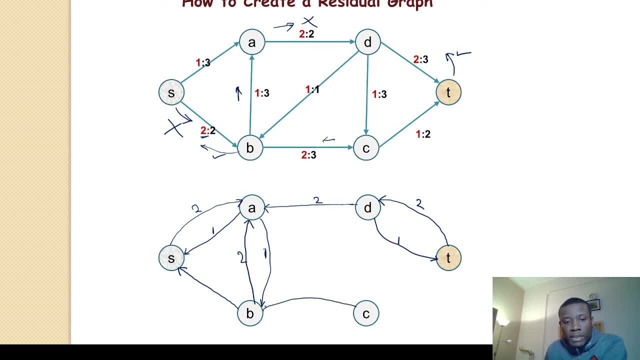 So backward edge from this time from c to b, right, and we have a forward edge of one because we need one more to complete it, so we can add one more in the same direction. so this is one in the same direction and this is two in a backward direction, right, good, so let's consider c to t, consider c to t. we have one. 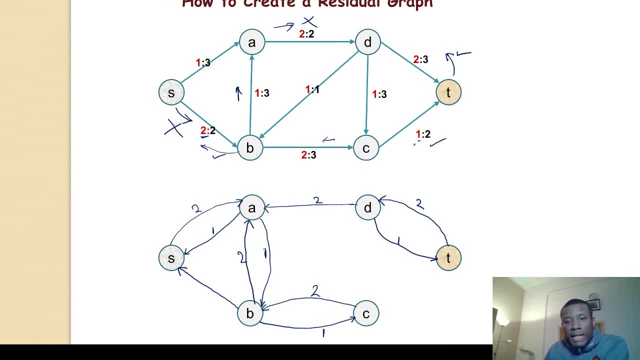 meaning that we can add one more in the same direction and we can add one more, we can add one backward edge to remove this traffic of one. so we have a forward edge of one and a backward edge, a backward edge of one as well. so we are left with d to c and also d to b.